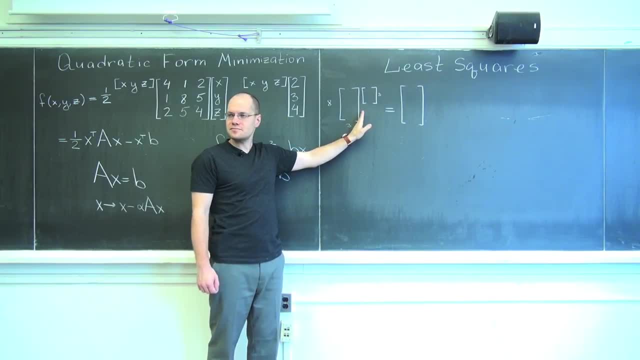 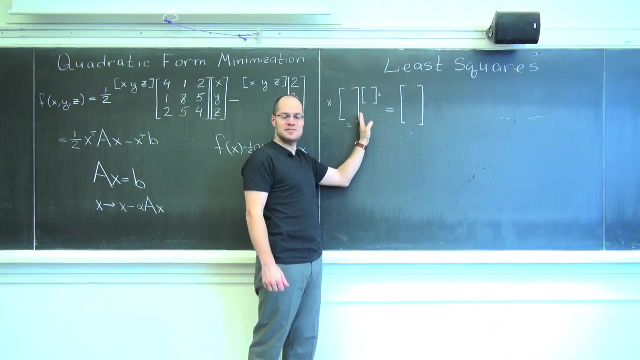 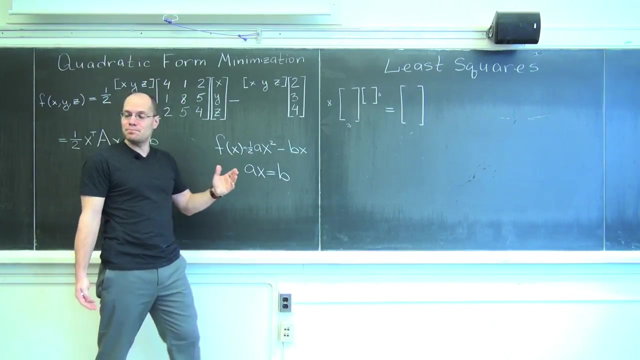 we only have 3 columns. We only have 3 columns to span an 8 dimensional space. Of course it will fail to do that. It's 5 dimensions short. So what are the chances that our target vector is in the column space of these 3 columns? No chance. So from that perspective too, there. 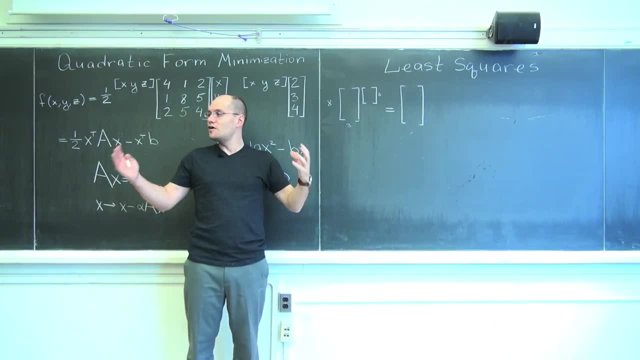 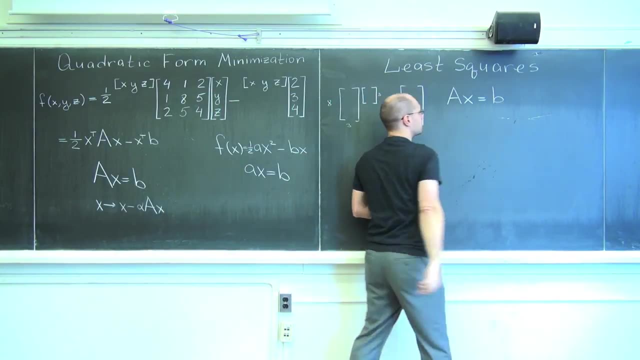 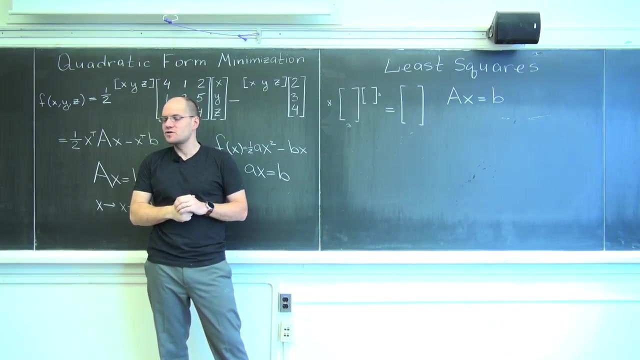 is no solution. So what are we going to do? Give up? Of course not. Here is what we'll agree on. Let's call this AXB, of course. Okay, This cannot be satisfied exactly, But maybe we will find the X, so that the discrepancy is as small as. 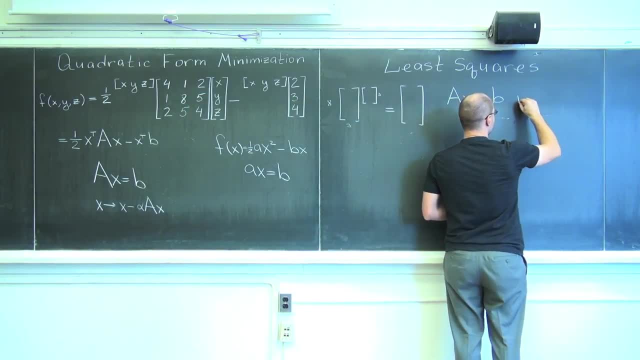 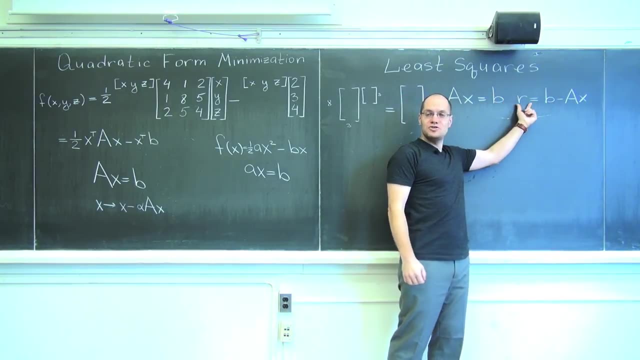 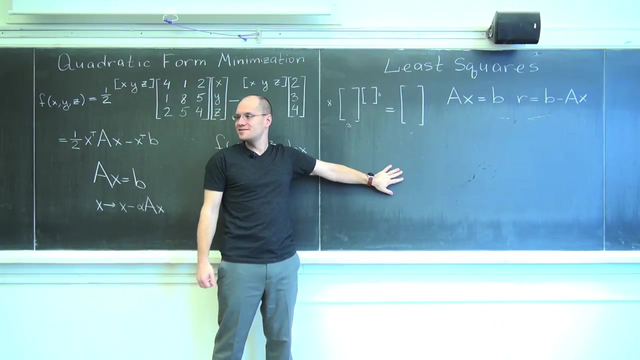 possible. We'll call it- I think R is a common R equals. I'll call it B minus AX. We want R to be as small as possible. So what this will end up being in just a moment is an exercise in matrix algebra. Some call? 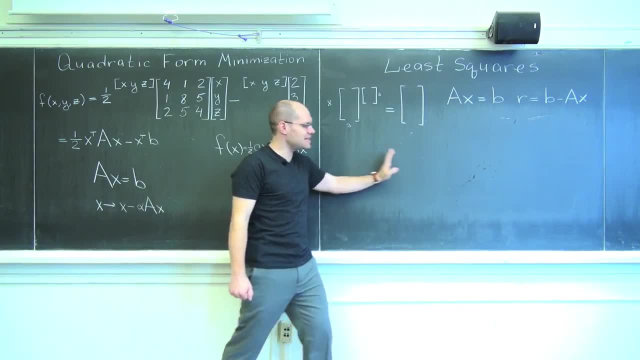 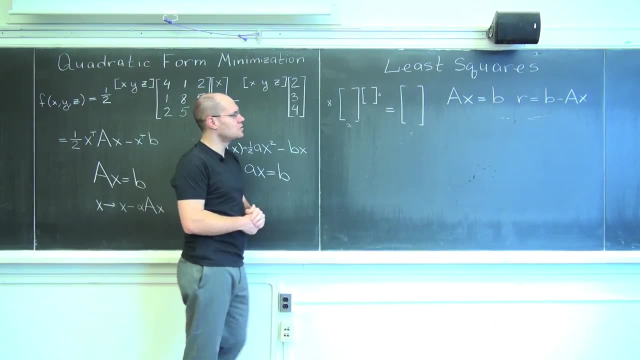 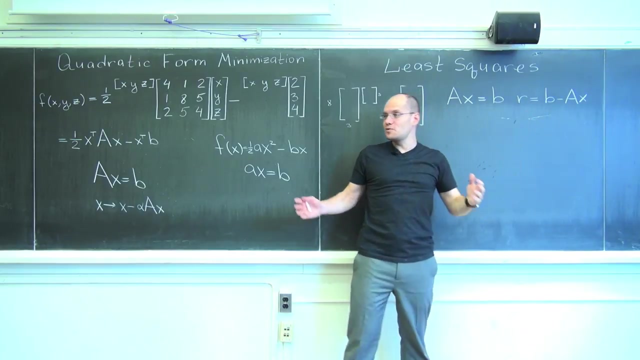 it matrix gymnastics. I think I would say this is as complicated an example of matrix gymnastics that you should be able to handle You'll see. Okay, So we want R to be as small as possible. Are you guys with me? So, before we started, embark on studying the third pillar, 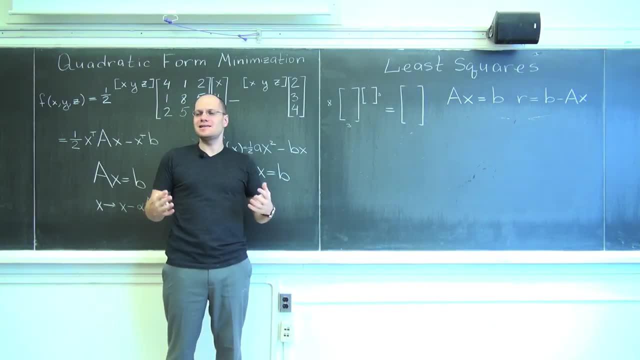 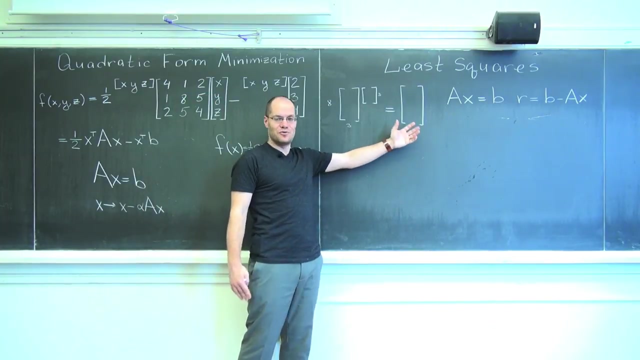 the third pillar of linear algebra. we were completely unequipped to even approach this problem because our vectors did not have length. our geometric vectors had length, but that's it. Our polynomials did not have length, and least squares over functions play a monumental role. 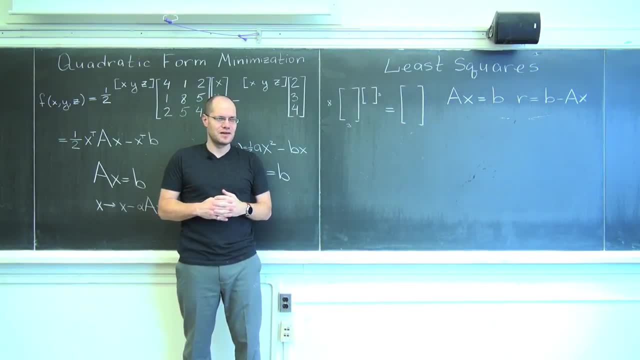 And even our elements of Rn did not have length, And if you thought they did that, I did the best I could to stomp it out, Stump it out, stomp it out, stomp it out, Yeah, stomp it out. 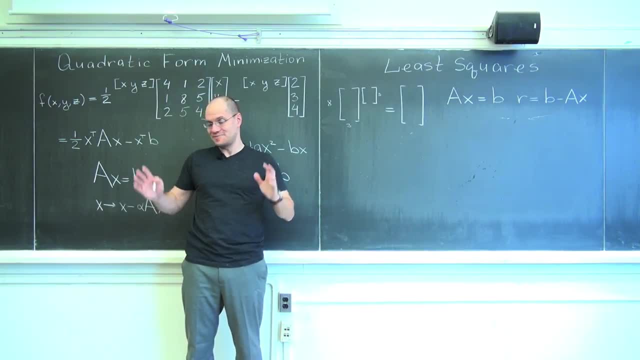 I forbade you from talking about lengths of vectors because you had to treat them on their own terms until we got to inner products. And now, with the help of an inner product, all of our vectors have length, as long as you introduce an appropriate inner product. 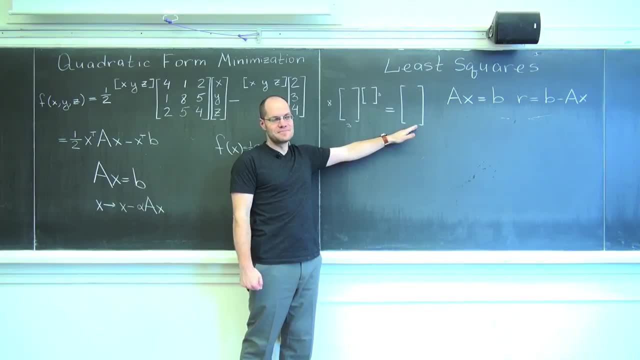 So what would be an appropriate inner product here? Well, you can use any inner product. Maybe the problem that this came from would dictate what the best inner product will be And, depending on that inner product, the math that I'm about to show you. 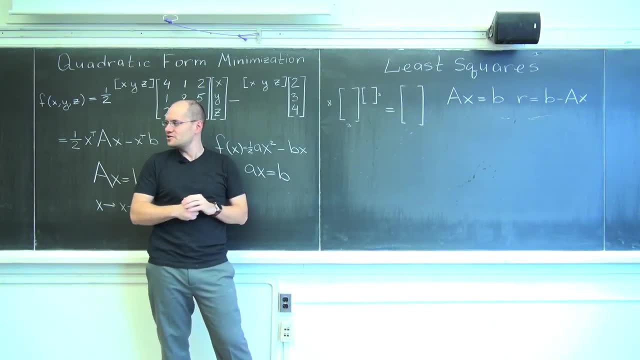 will be just a little bit different, would have a little extra ingredient, So I will use the standard inner product, much to my chagrin. But once again, we're not trying to. we're trying to illustrate a particular thing, so it's okay. 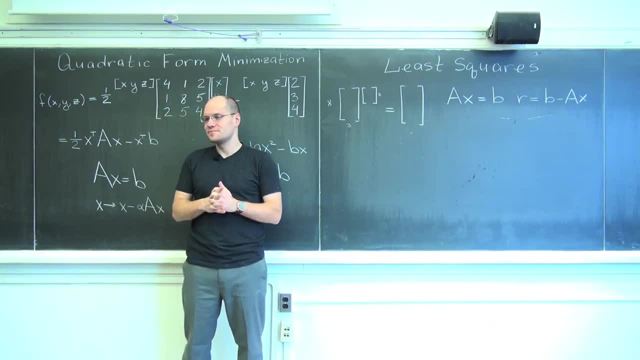 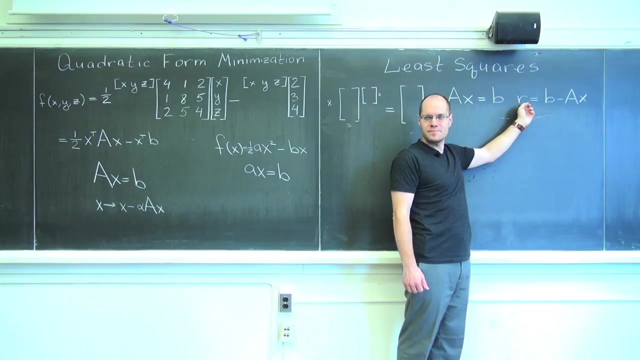 You know we'll go back to our general inner product soon enough, maybe in the next lecture, probably in the next lecture. So yes, we will use the standard inner product And, with respect to the standard inner product, this is an element of Rn. here's what makes our R8, Rn. 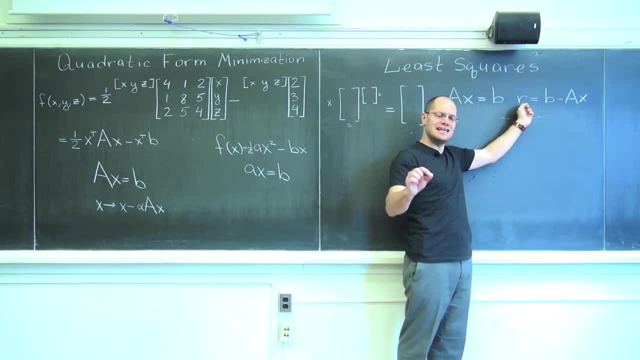 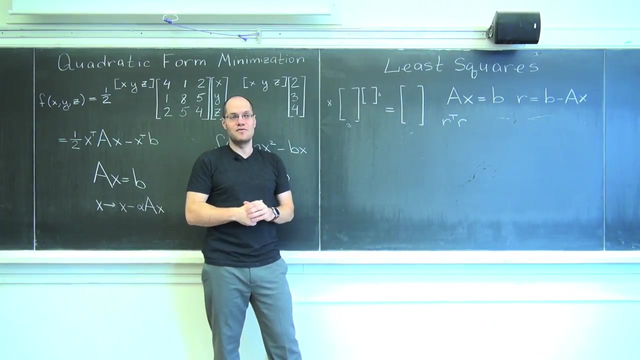 Here's what makes the standard inner product nice. It is particularly easy to express in terms of in the language of matrix algebra. Be careful, Because the length of R squared is just R transpose R. Are you guys with me? What is the length of R? 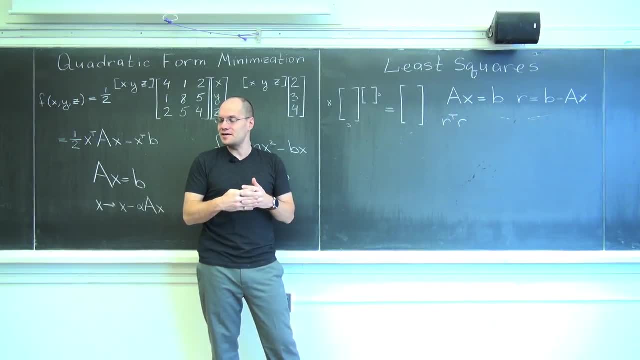 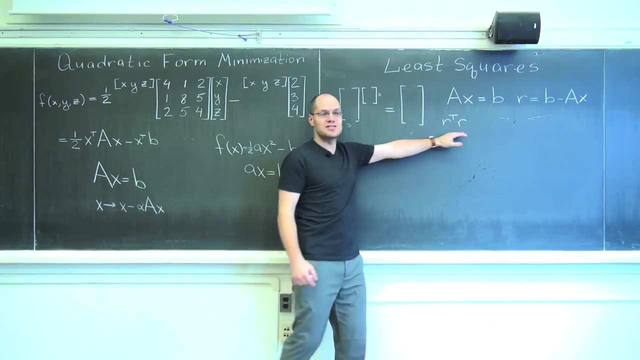 You dot it with itself. What does it mean to dot with itself in the standard inner product, The sum of squares of the entries. What's the matrix notation for it? R, transpose R. So I think we just sorted it all out, right. 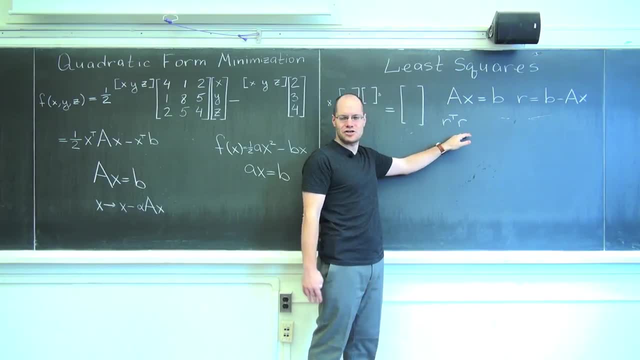 So it would be wrong to say that the standard inner product is defined as R transpose R. no, It's just matrix. It's a matrix expression for it. I think we learned today because this exercise took all of you 15 minutes on average. 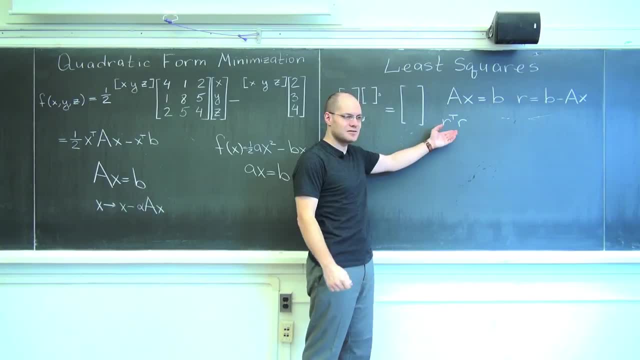 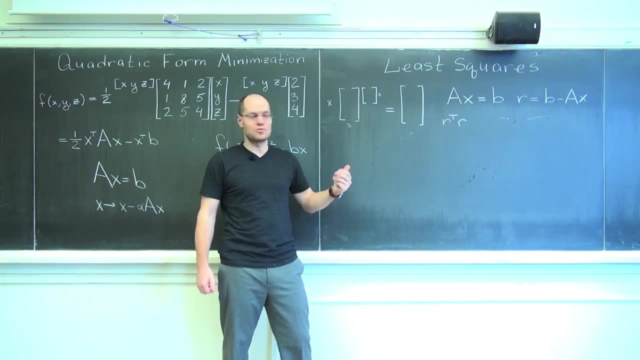 right that matrix notation is not always best, But it's good here. so we're going to use matrix notation. Okay, R transpose R. So we have our starting point and now we can roll. Let's plug in what R is. 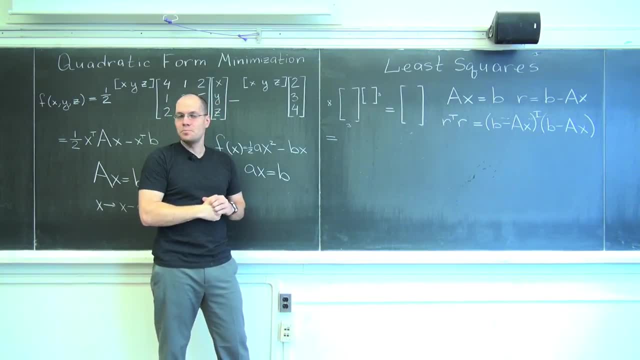 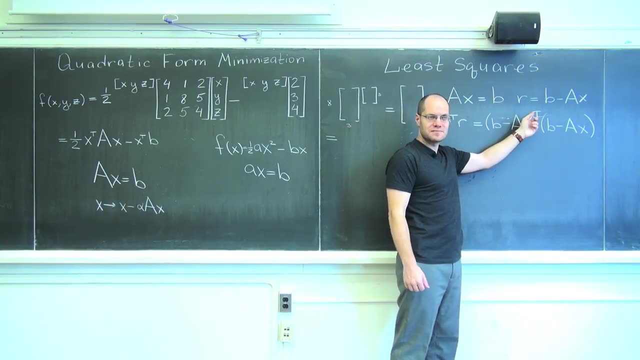 So you see foil coming out right, Foil will happen, But first the transpose will happen. So we need to take this difference and transpose it. Of course it's the difference. Let me call it sum- Sum. It will be the sum of the individual transposes. 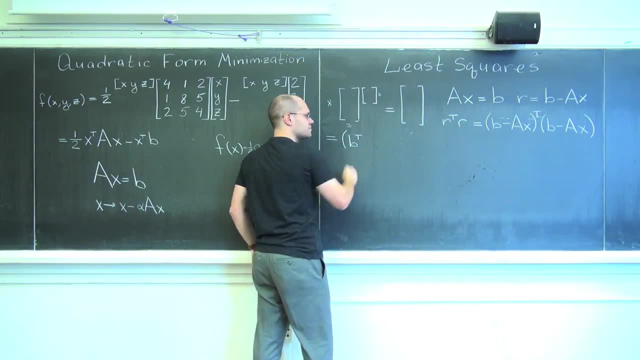 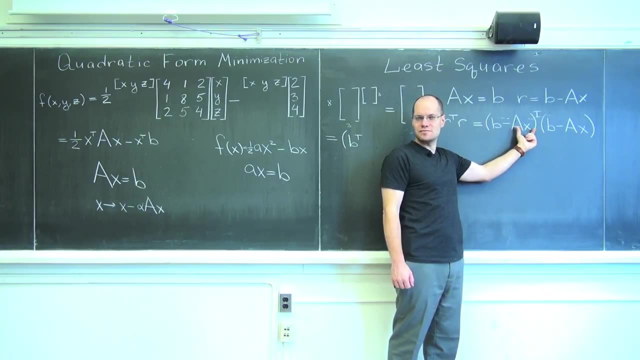 so it will be B transpose. Okay, but this is the transpose of the product. AX transpose, Which, you're exactly right, is the product of the individual transposes in the opposite order, And it just I always marvel in mathematics how saying it really helps. 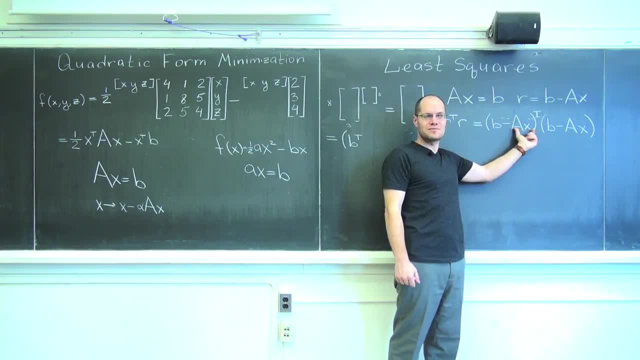 but hearing it doesn't help at all. It only helps it when you say it yourself. When somebody says: oh, the product of the, the transpose of the product is easy, It's just the product of the individual transposes in the reverse order. 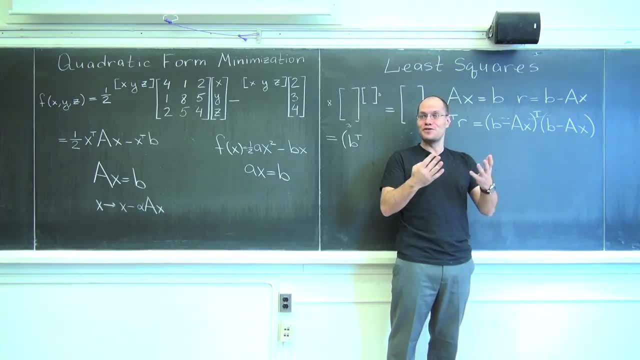 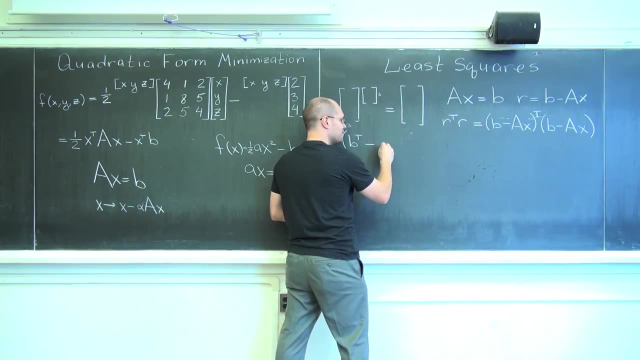 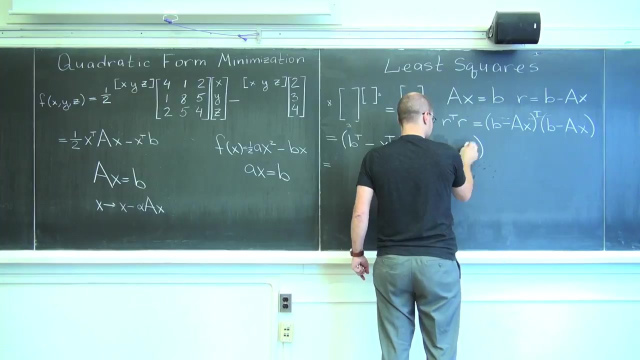 That's not helpful. But when you look at a formula and you verbalize it yourself for some reason, that's very helpful. So I always hesitate to say that. but that's what it is: B minus AX. Okay, going on to the next line. 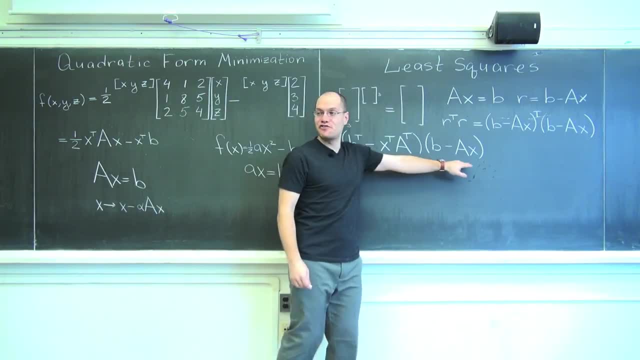 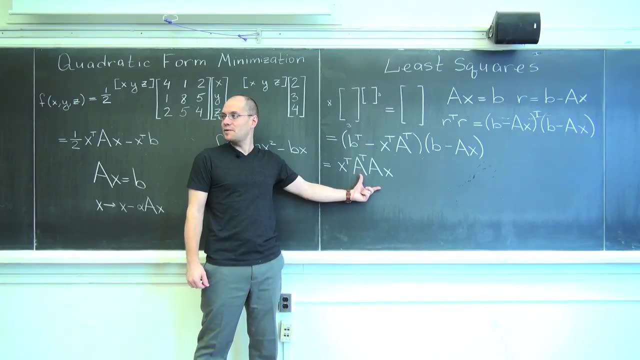 Let me foil it in the order that I want. I'll take the last ones first. Now we see a combination. we've seen before A transpose A. I promised you that you would see this sort of combination all the time, and of course you do. 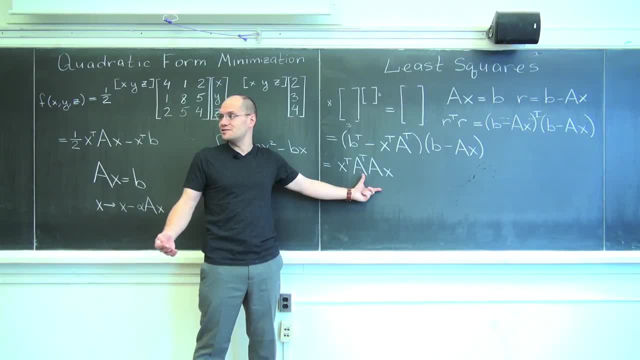 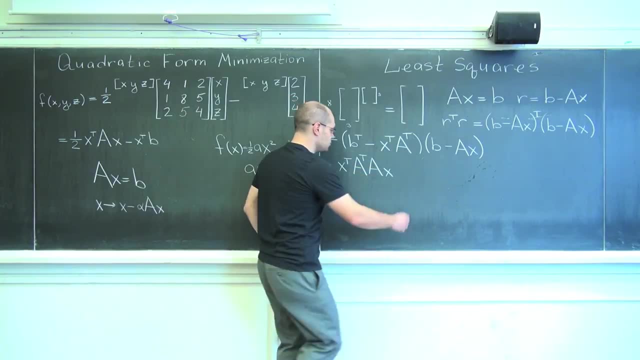 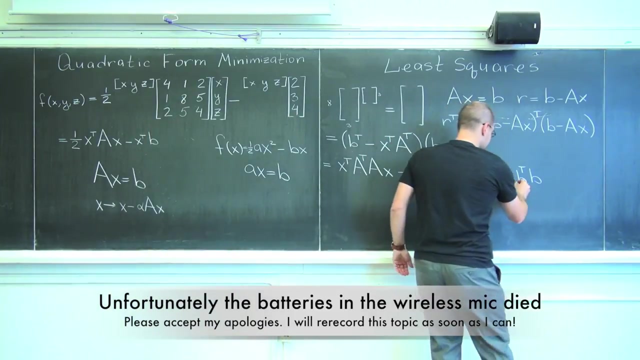 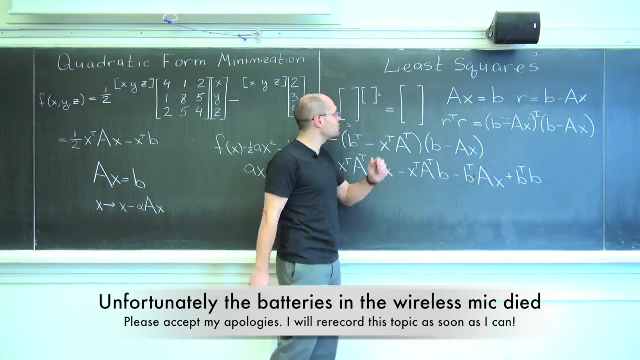 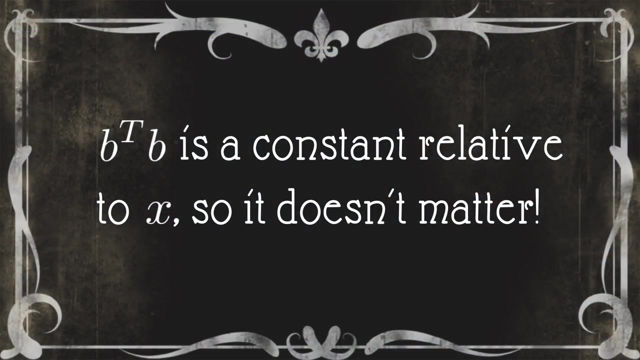 You always have it when you dot things with each other that involve matrices. Okay, good, Minus X. transpose A, transpose B. Now you can see that I have to split it out to show it in the way that A transpose B would, so you can see the differences. 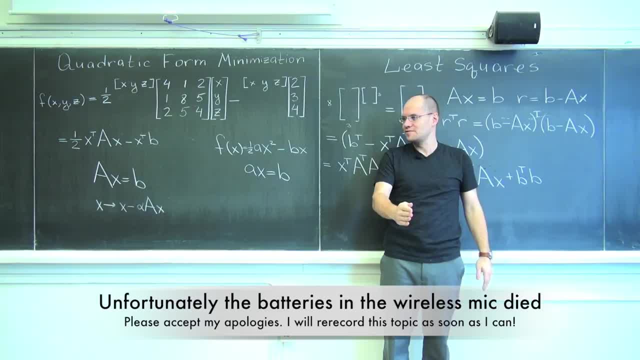 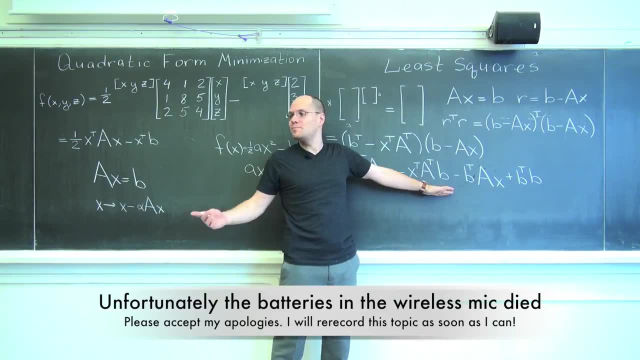 The difference between A transpose and B transpose is that there's an aftertan. You can see that they're going to be in the same order. Well, let's see with two: One transpose B two. So A transpose, B two. 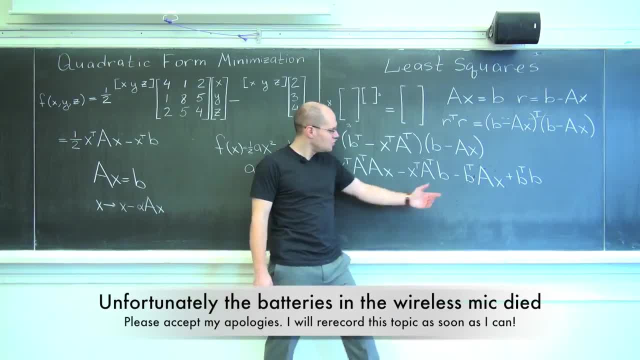 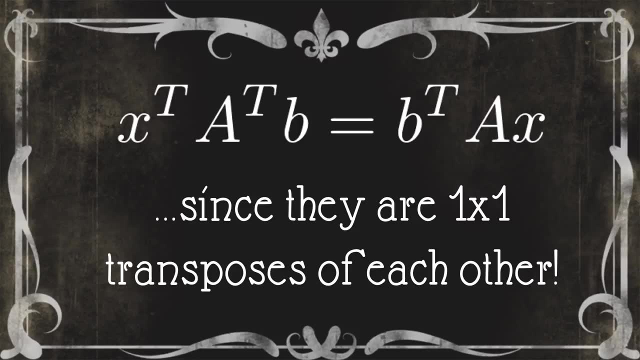 One transpose A transpose B two. There's the difference. So you take the first one. Two transpose B Two. zero rs, Two zero rs. You take the next one. Four transpose B two. four, Two, vier, four cube four.